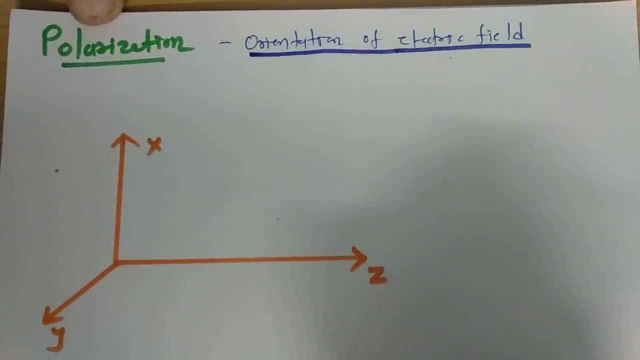 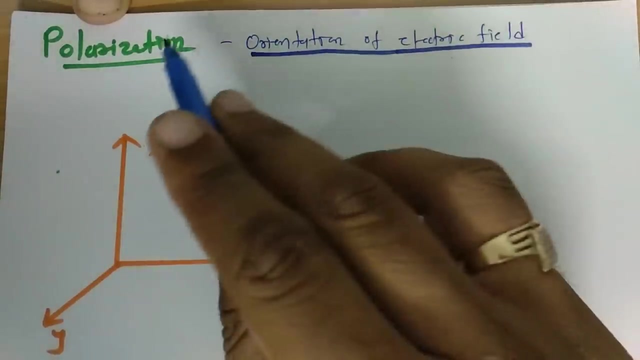 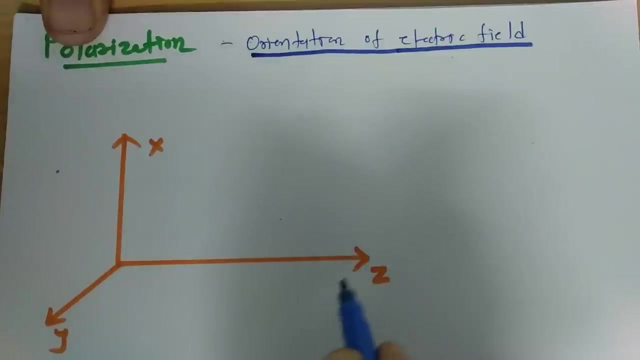 So before I explain how to understand what is polarization of electromagnetic wave, I will explain first of all how electromagnetic wave propagates. So here I will be showing only electric field to understand polarization. So here, if I say I have electromagnetic wave which is propagating along with z direction and its orientation is associated with respect to x-axis, 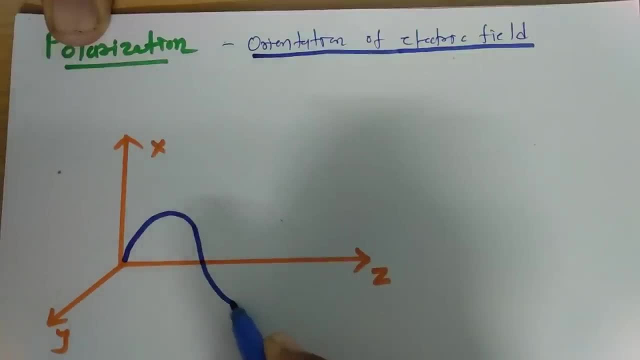 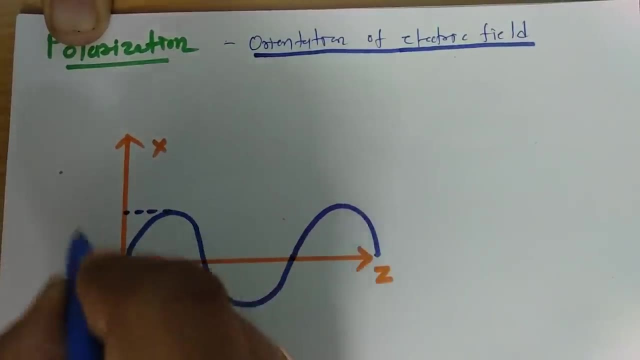 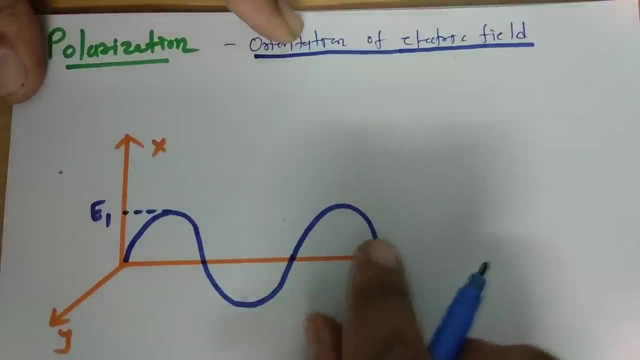 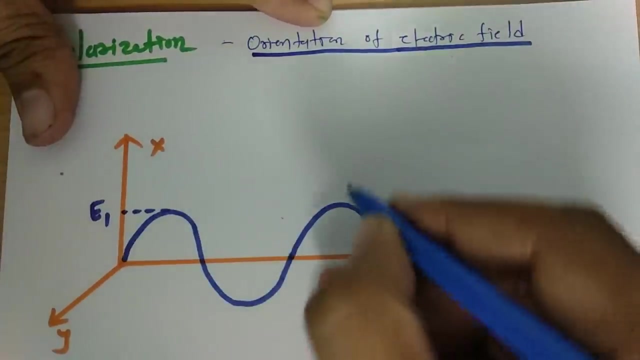 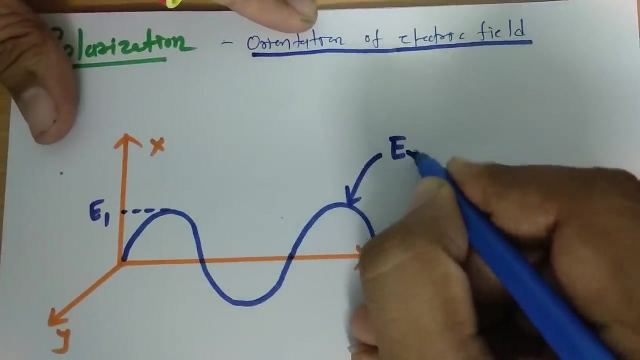 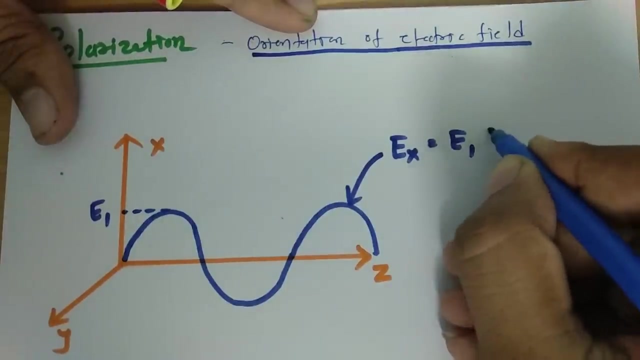 So if electromagnetic wave that is propagating like this and its maximum amplitude with respect to x, that is e1, then this electromagnetic wave that is having polarization with respect to x-axis, and to explain this we can write this electric field by ex, and that is maximum amplitude, is e1- into sine omega t minus kx. So that is how. 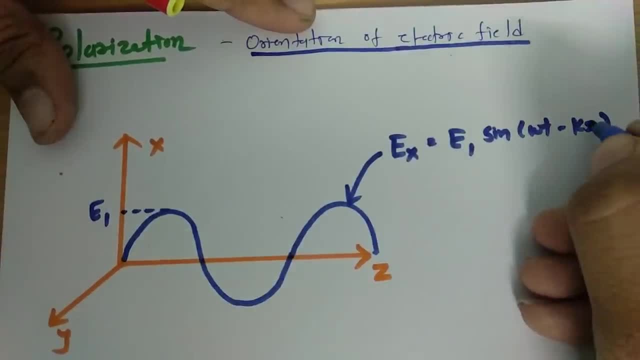 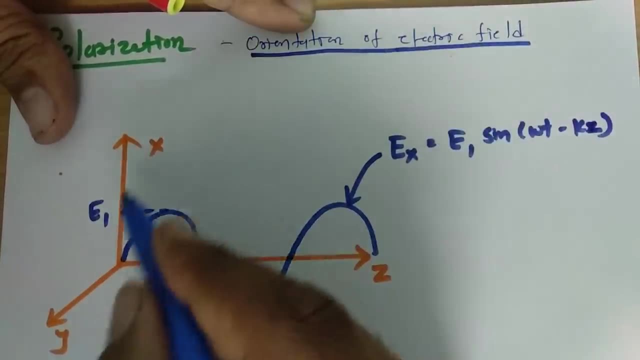 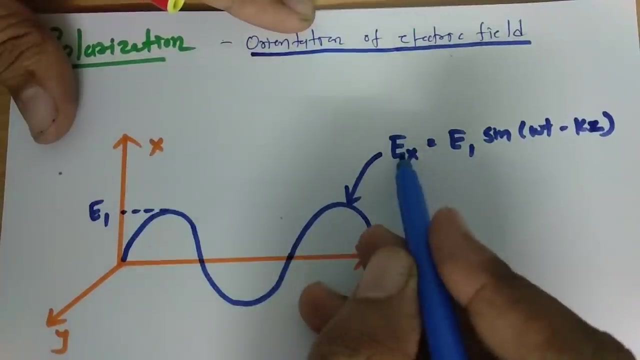 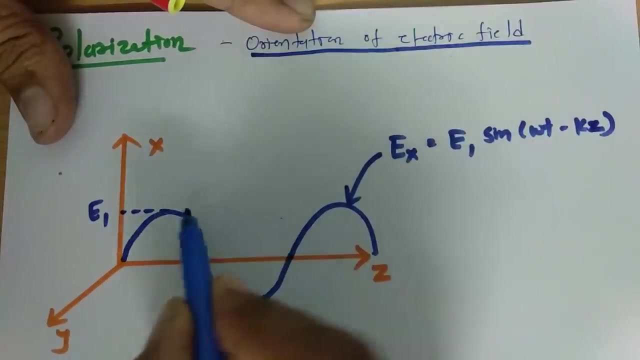 sorry, here it is propagating along with z direction, so it should be sine omega t minus kz. So electric field along with x-axis, that is, ex is equal to to. electric field is associated with x axis. that's why electric field is with respect to ex only and that will be e1, which is what maximum amplitude with respect to x axis. 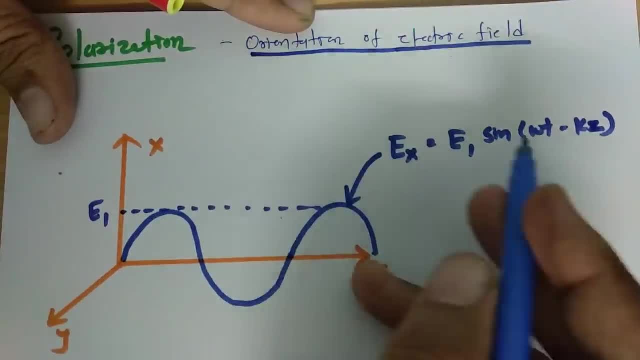 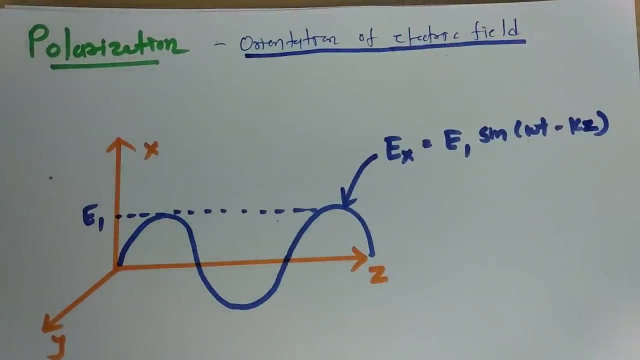 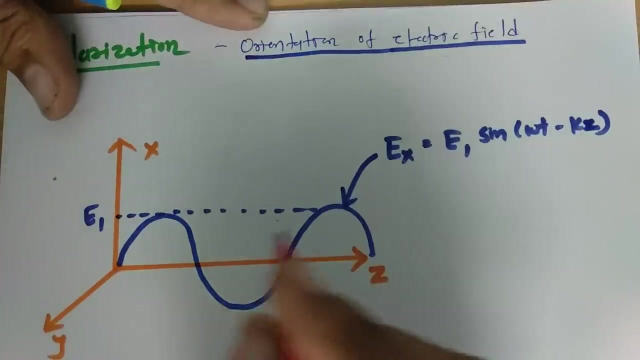 and omega. t. omega is frequency of this electromagnetic wave, and kx kz, where z is direction of propagation. so that is how one can write this formula of electric field: if electro electric field is propagating along with z direction, like this. now there could be a second way by which one can understand electric field, like for example: 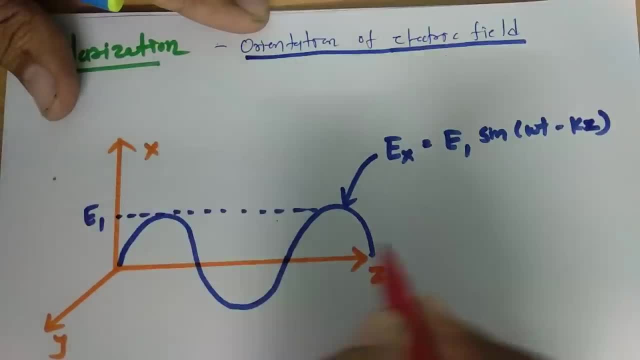 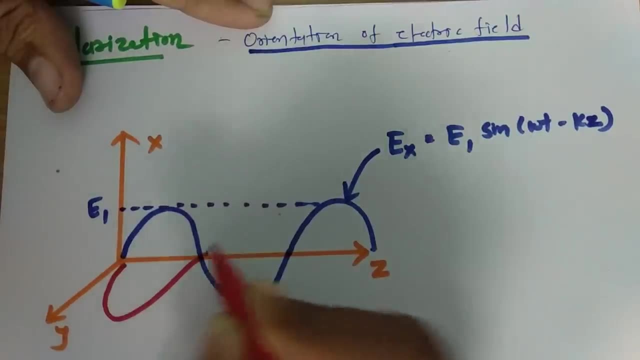 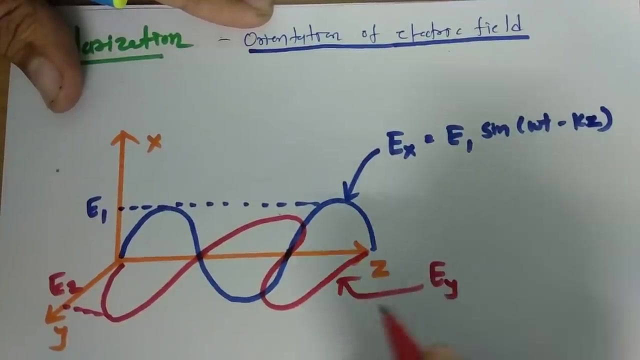 if electric field is propagating along with z direction and orientation is there with y axis, as i am showing it right now, like electric field is varying like this along with Y axis, and if I say maximum amplitude is E2, then electric field of this that could be explained by EY. the reason is electric. 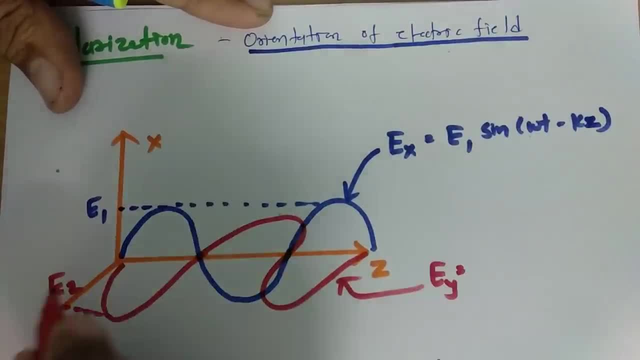 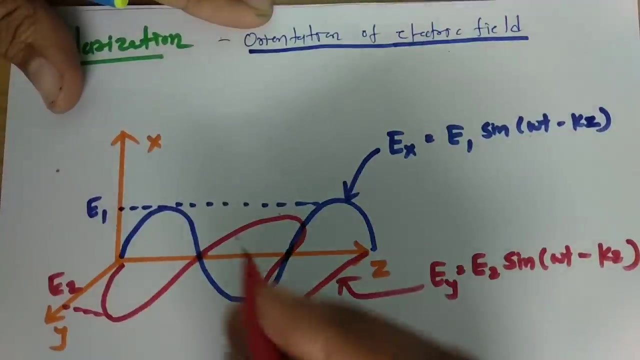 field is there with respect to Y axis, and that is maximum amplitude, is E2. so E2 sine omega, t minus kz. so here one thing is very clear: I have shown two electric field waves. one electric field that is there with respect to x axis and direction of propagation is 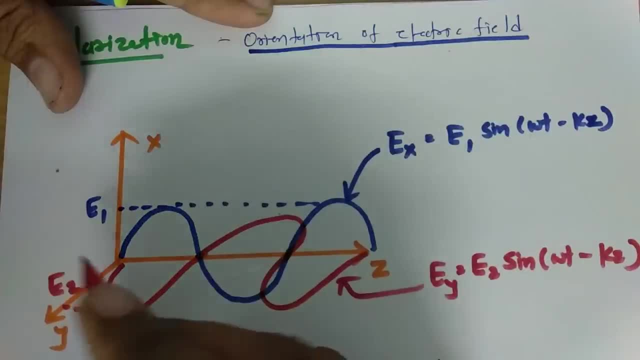 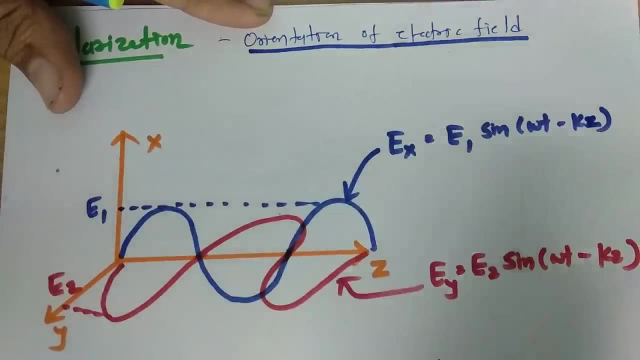 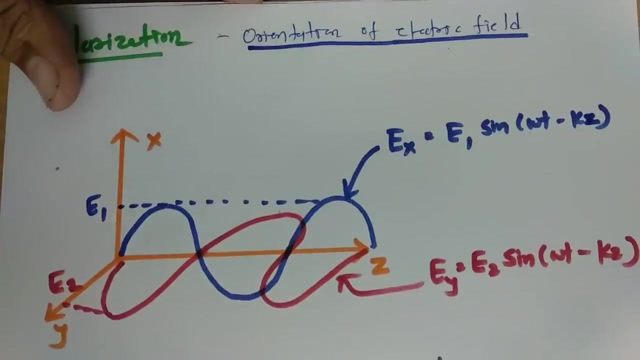 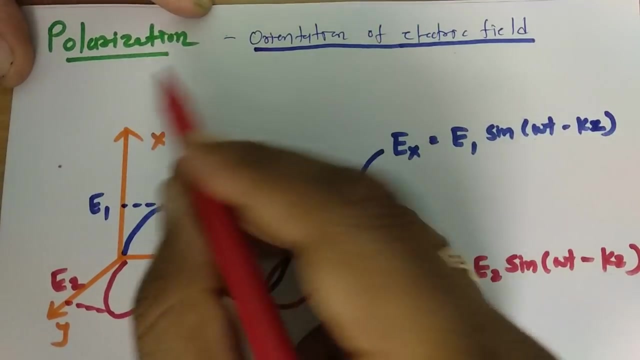 there in z direction and second electric field by red line one can see that is varying with respect to y axis and direction of propagation is in z direction. so that is how electric field that I have shown over here now to understand what is linear polarization. so, as I have explained, polarization is orientation of electric field. so in linear polarization, 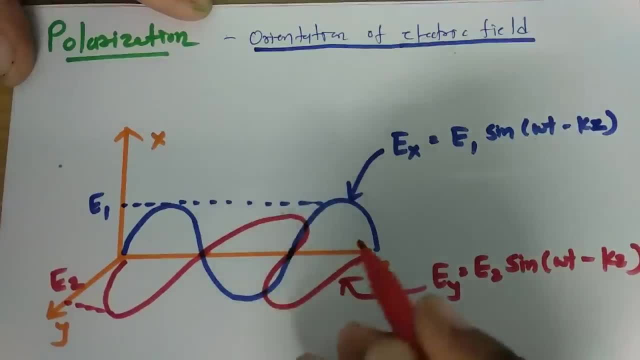 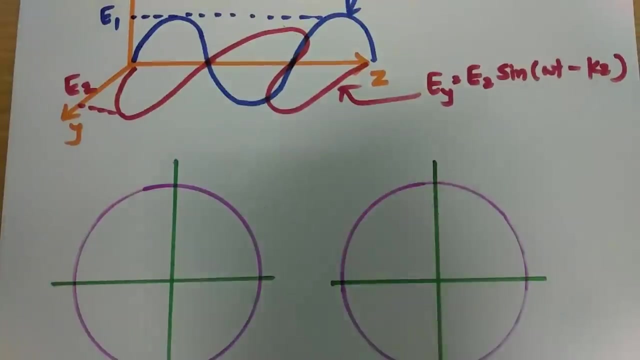 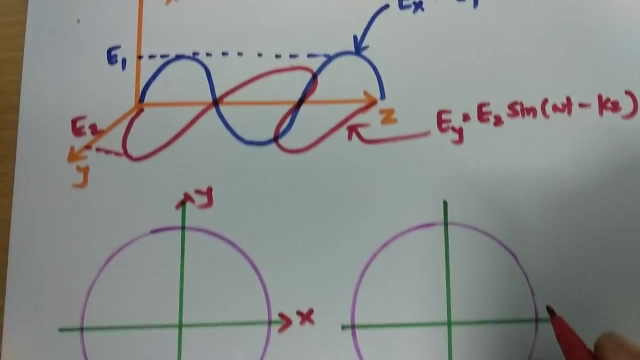 orientation of electric field is there with only one axis. so either you can see that I have shown two electric field that is there with respect to y axis, or electric field will vary with respect to x axis, or it will vary with respect to y axis. so here I will show it like: see, this is what x axis and this is y axis, and as by blue color. 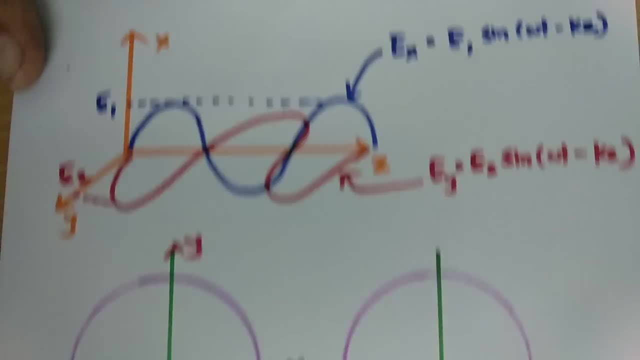 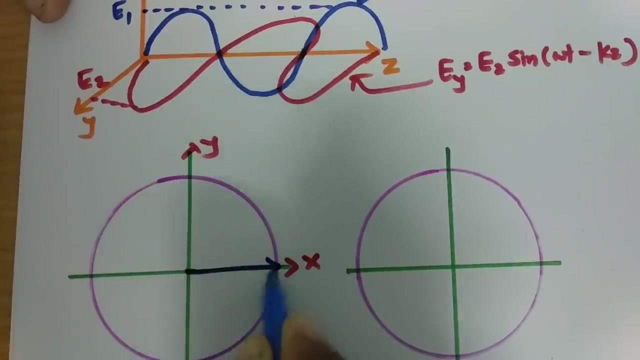 I have shown, electric field is varying with respect to x axis. so for this blue color line polarization, then it will vary with respect to y axis. so here I have shown two electric field that is there with this direction. if I say this is origin and direction of propagation, that is there associated with z direction, so that 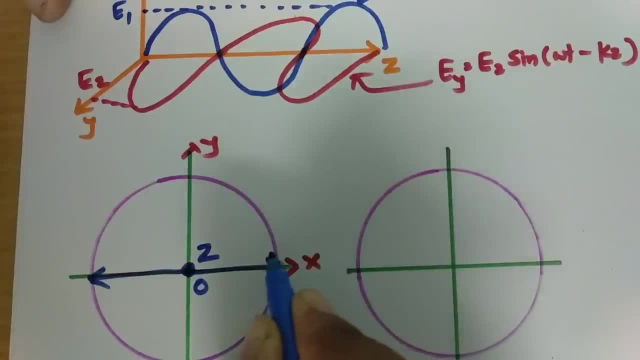 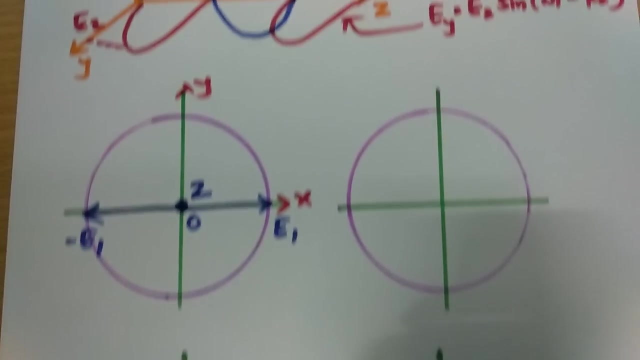 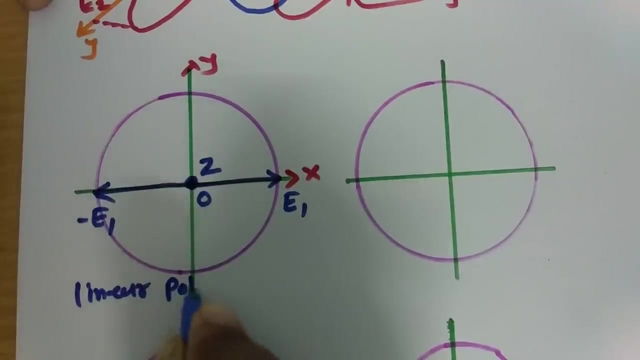 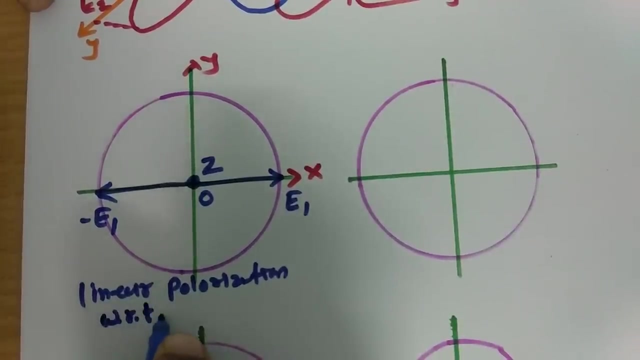 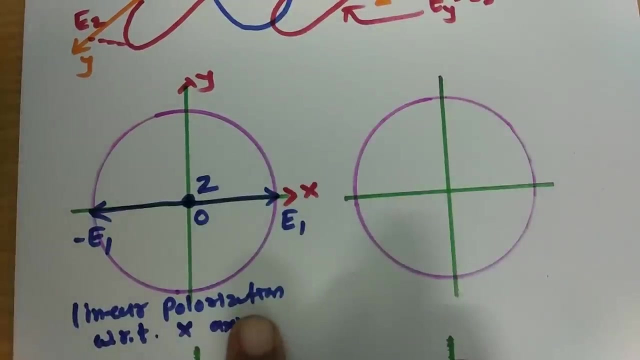 is there inside the page now either. it could be plus e1 here. it could be plus e1, here it could be minus e1. so it is associated with only x axis. so this is what linear polarization with respect to x axis. so this is linear polarization to be with respect to x axis. 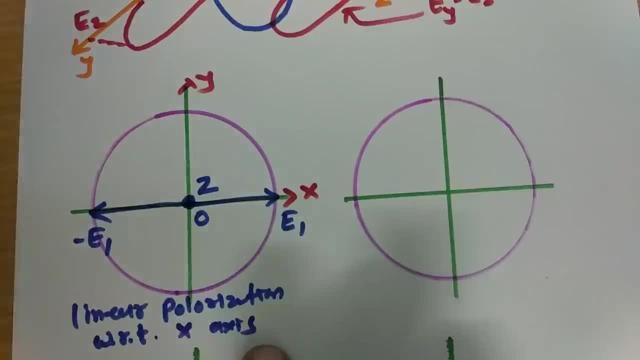 so what is linear polarization? linear polarization is orientation of electric field. is there along with x axis or y axis, or a non selecting field vector with respect to y axis in the axis? it should be there with only single axis. in short, Like, if you want to understand this, 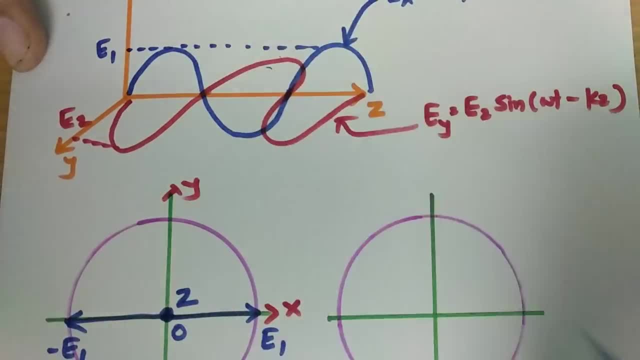 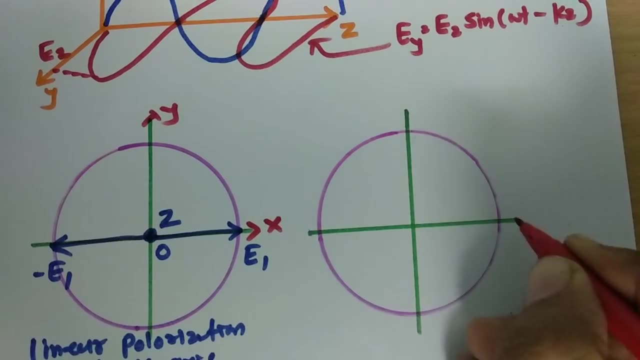 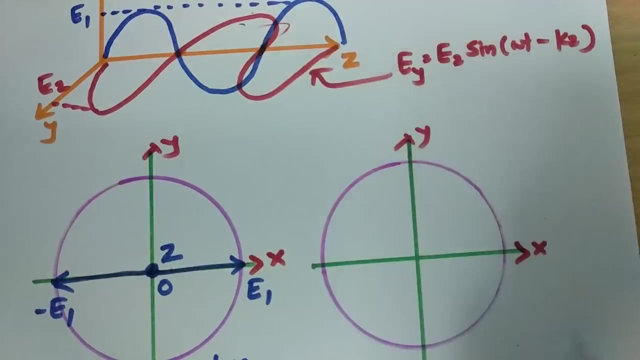 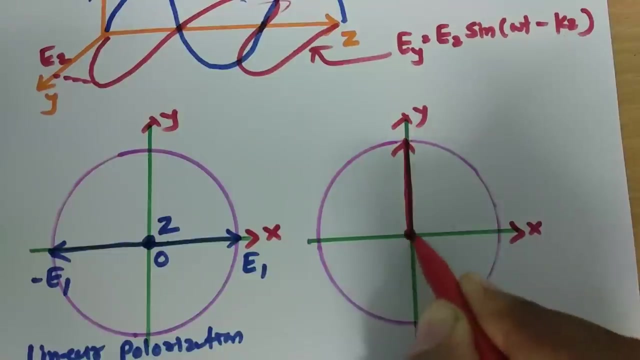 with this red color polarization, then for this red color polarization that is along with y axis. So if I say this is x and this is y, so this signal of electric field that is varying with respect to y axis, So electric field that is varying like this where here it is getting, 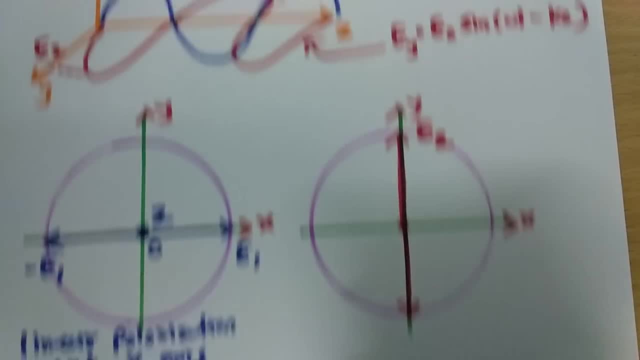 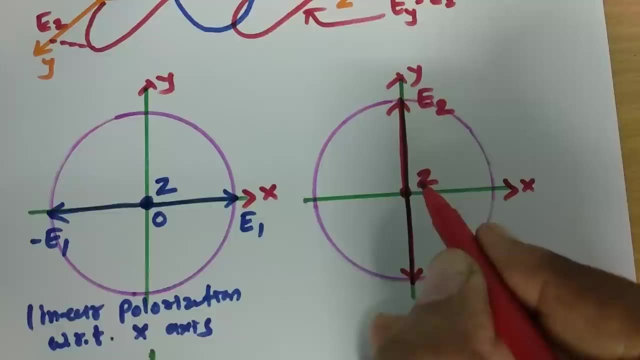 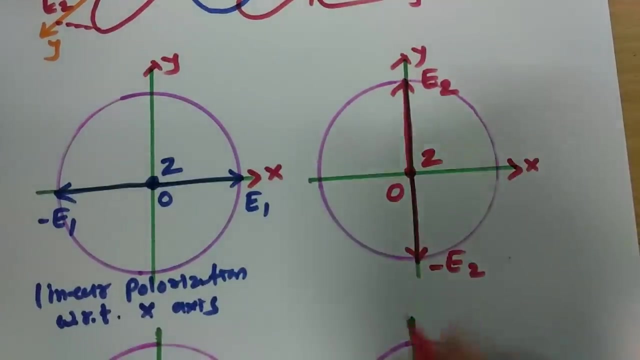 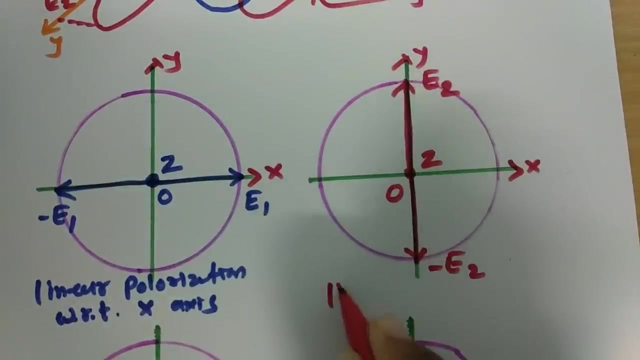 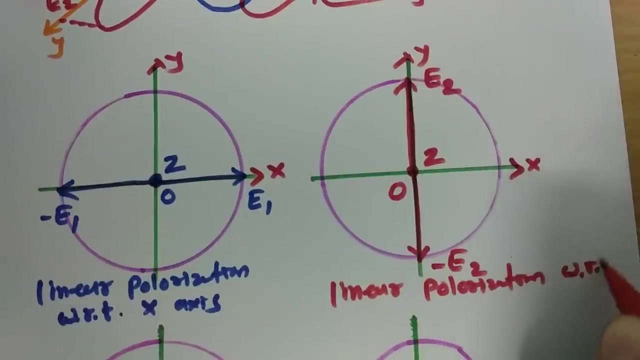 E2. maximum amplitude, that is E2 or over here it could be minus E2. and direction of propagation. that is there along with z axis. I have considered it is inside the page. So direction of propagation is there inside the page. So this is what. linear polarization with respect to y axis. This is linear polarization with respect to y. 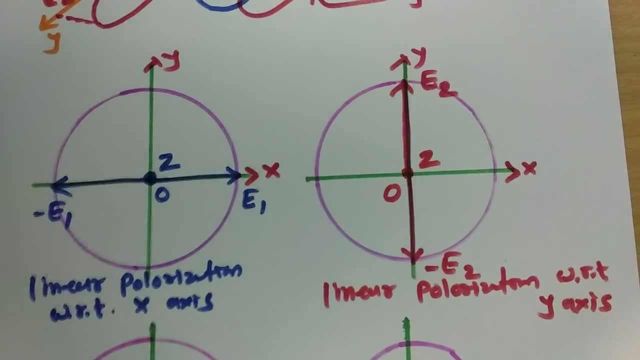 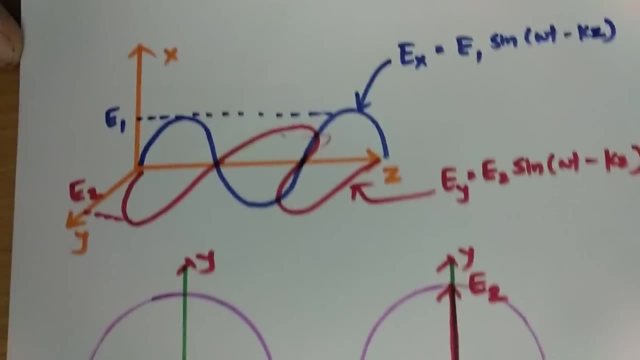 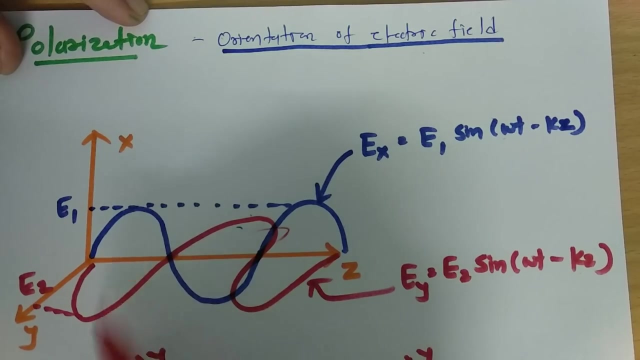 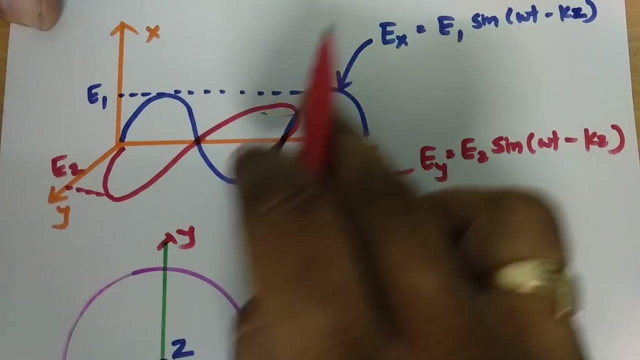 axis. So that is how this linear polarization is there with respect to y axis. So what is linear polarization? Linear polarization is orientation of electric field with respect to one axis. It could be there with respect to x axis, which one can see. this is what with respect. 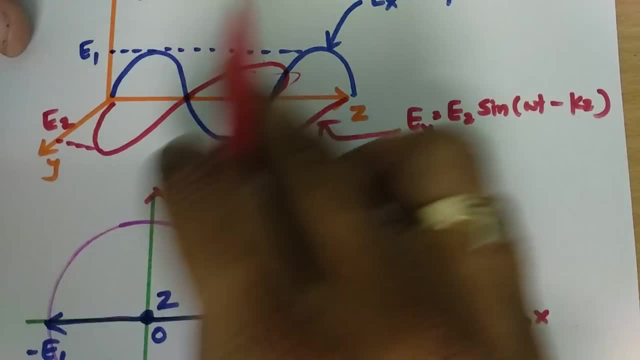 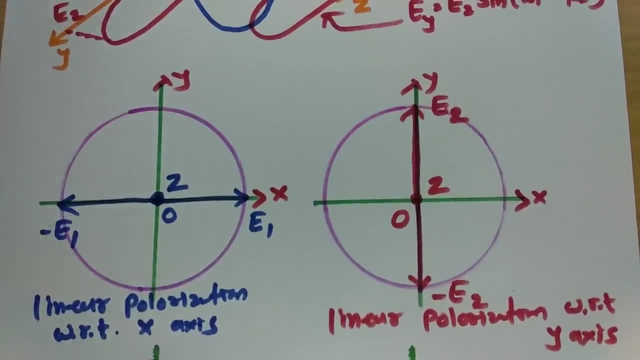 to x axis, or it could be there with respect to y axis, So it is varying only with respect to y axis. So this is what example of linear polarization. Now let us try to understand what is circular polarization. So in circular polarization, 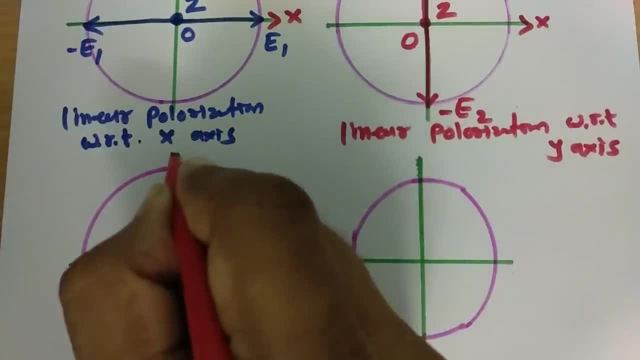 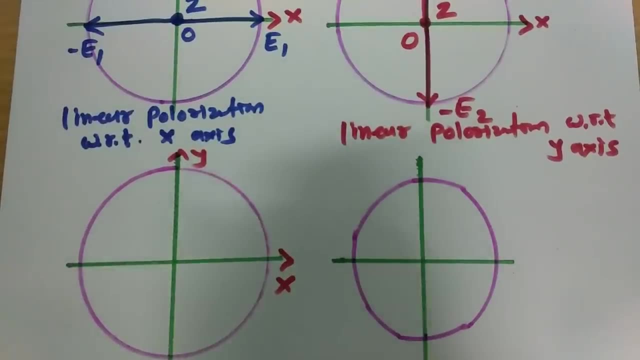 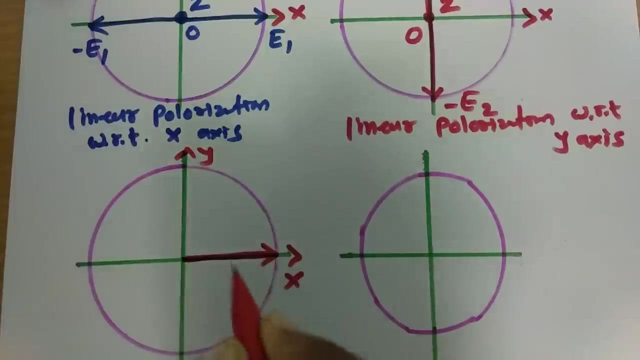 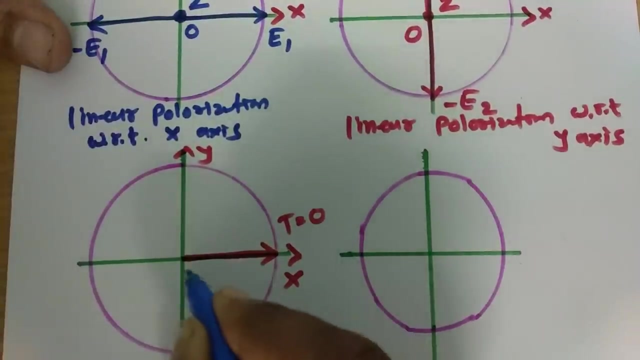 if I say this is x axis and this is y axis, So with respect to time, signal will rotate Like see: for example, if I say electric field that is there along with x axis, at time t is equals to 0. And now if electric field that is oriented in this direction after time t is, equal to 0,, then there is a suffering. So let us try to understand what is circular polarization. And now, if electric field is oriented in this direction after time t is equal to 0, then there is a suffering. So this is 60 times 0.. 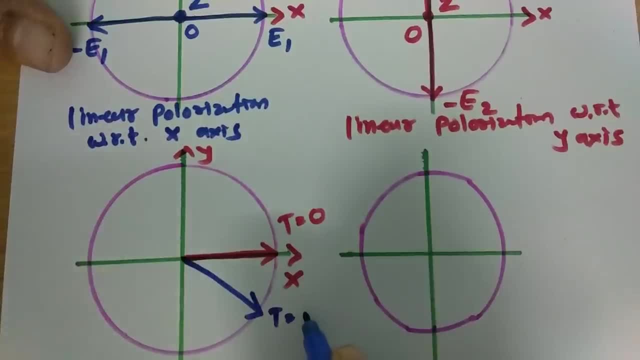 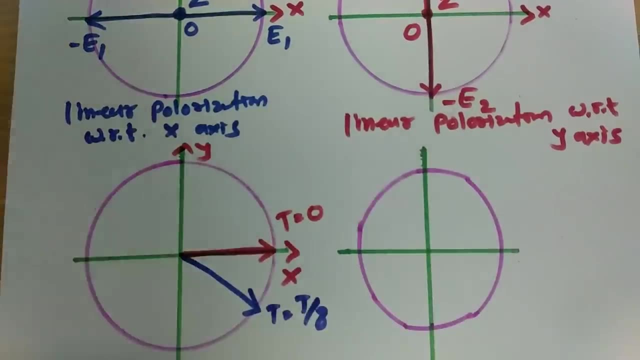 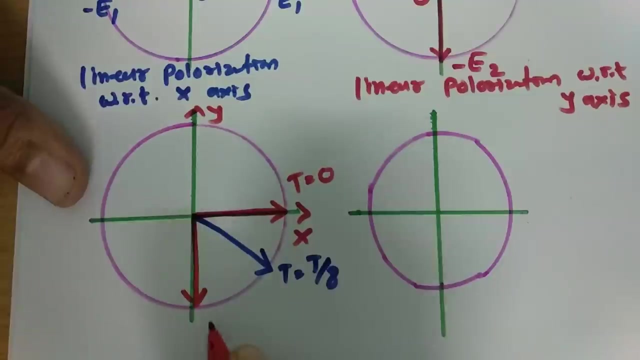 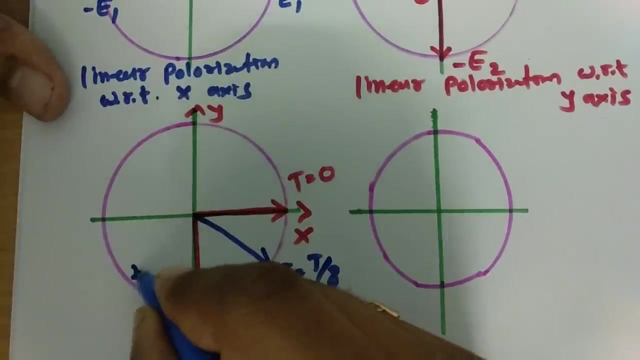 equals to, let us say, t by 8.. So at t by 8 it is over here Now after 2t by 8, this electric field that reaches over here. So after time 2t by 8 it reaches over here After time 3t by 8. 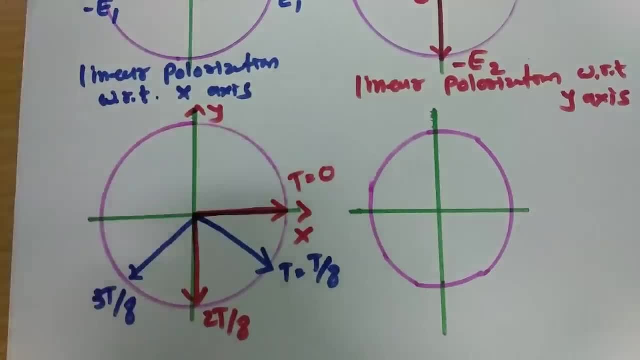 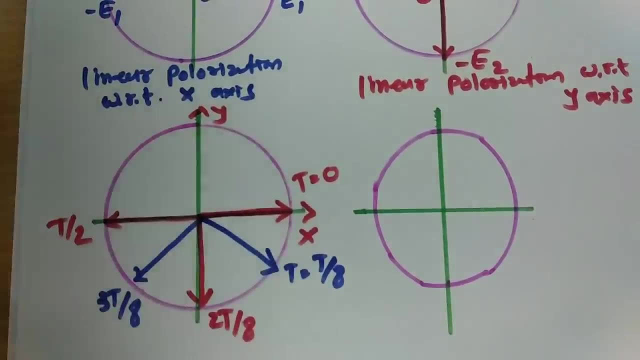 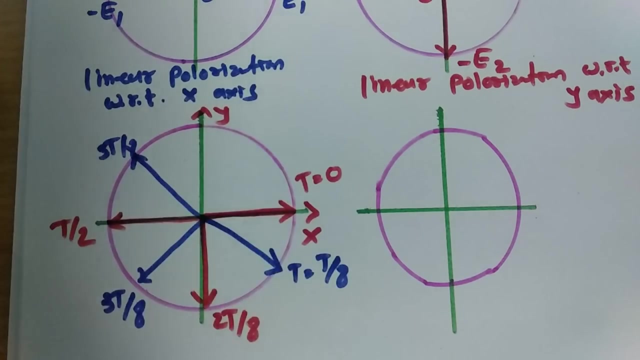 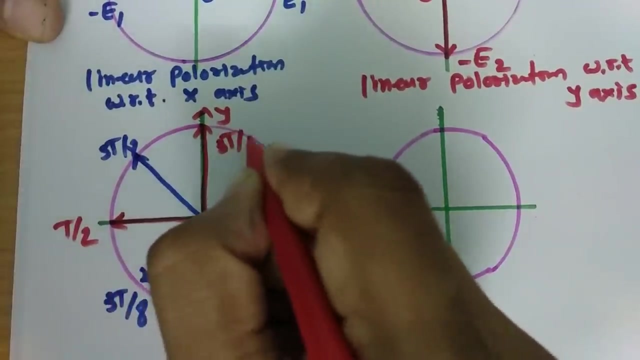 it reaches here After time t by 2, it reaches here After time 5t by 8, it reaches here After time 6t by 8. or one can say 3t by 4, it reaches here. So see, this is how electric. 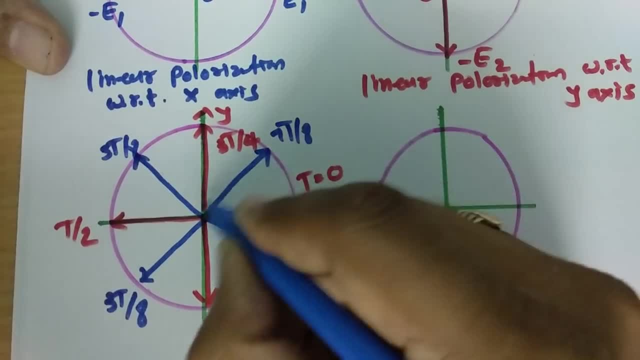 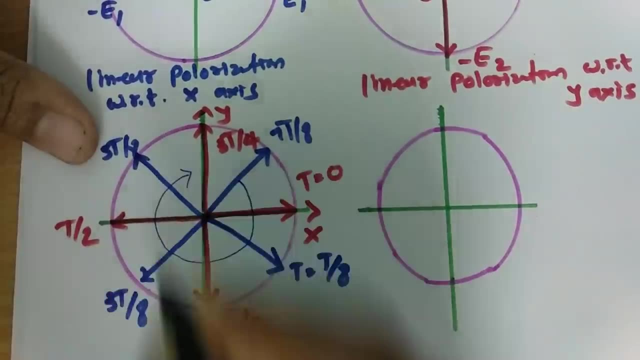 field reaches over here. So at t by 8 it reaches over here After time, 6t by 8, it reaches over here After time, 7t by 8, it is reaching here. So ultimately, electric field that is revolving in this direction. So this is what: clockwise circular polarization, This is what 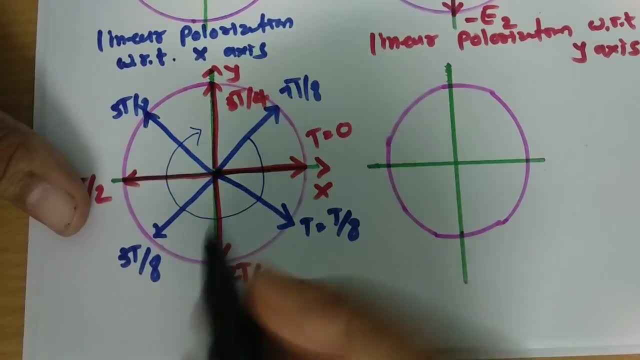 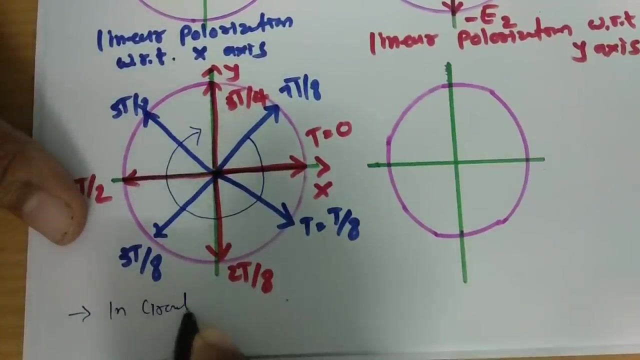 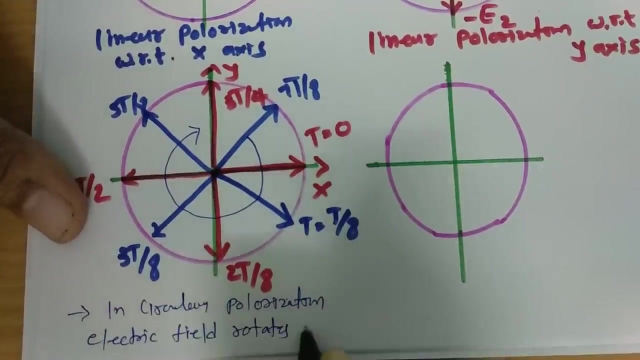 clockwise circular polarization, where electric field is revolving like this, with respect to time. So orientation of electric field that is getting revolved with respect to time, rotation with respect to time. So that is what circular polarization. So in circular polarization electric field rotates with respect to time. So when you have this kind of reason that the solar movement 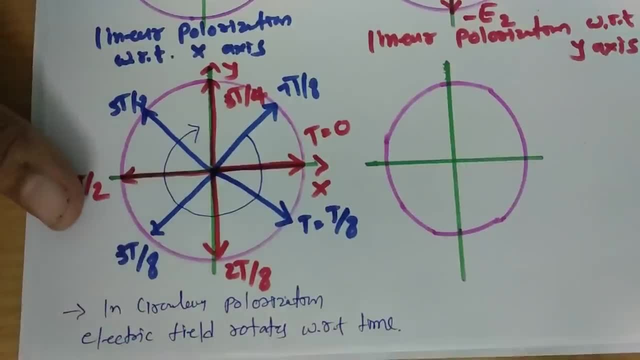 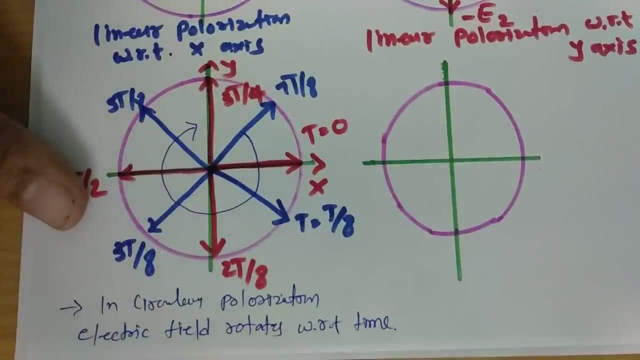 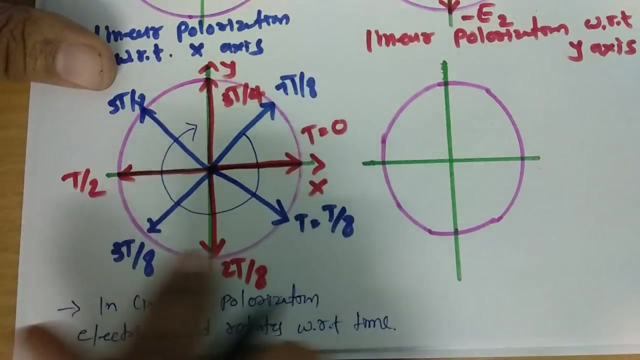 If it rotates in clockwise direction, then that is clockwise circular polarization, And if it rotates in anticlockwise, then it is anticlockwise circular polarization. But when we talk about circular polarization, magnitude of electric field along the axis will not change. 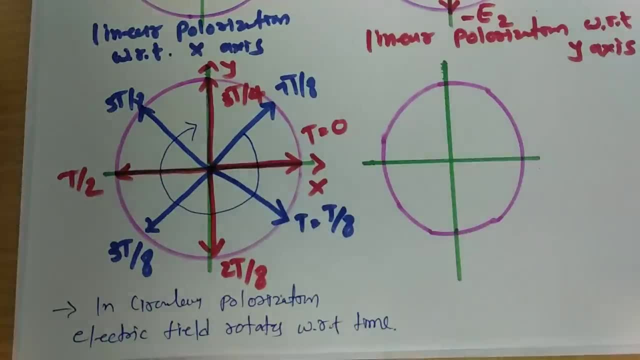 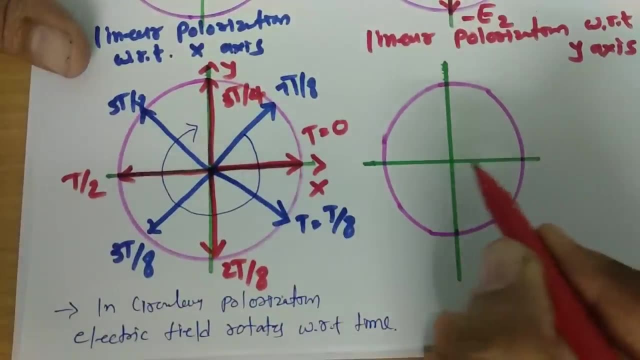 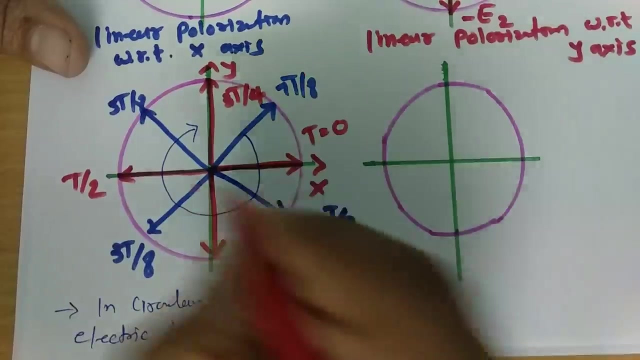 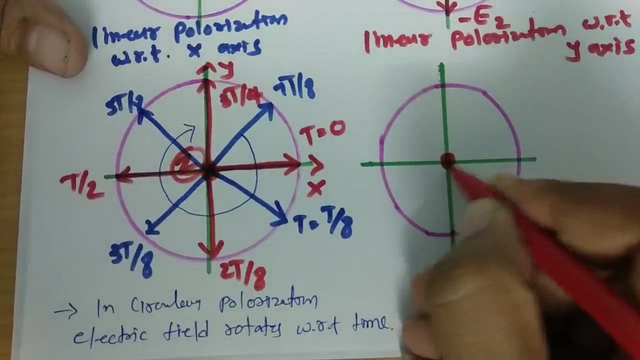 Now let us try to understand elliptical polarization. So in elliptical polarization electric field revolves with respect to time, But magnitude is different on x-axis and y-axis. Here, direction of propagation that is there along with z-axis, So here even, direction of propagation that is there along with z-axis. 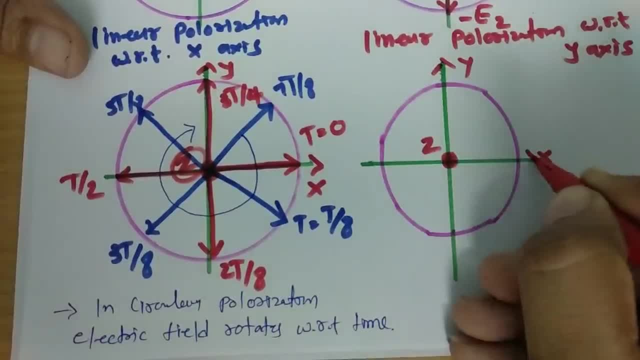 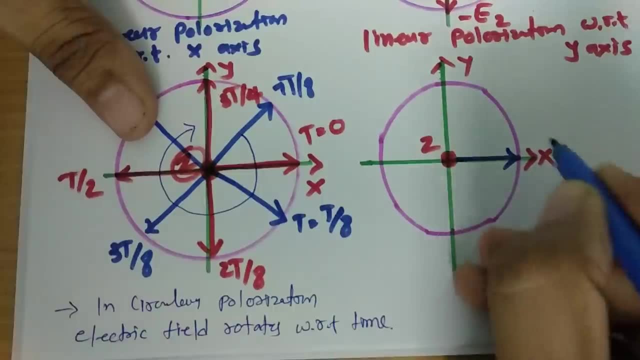 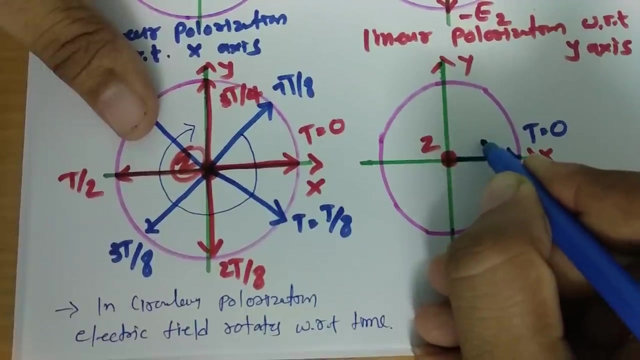 Let us say this is x-axis, this is y-axis, And now, If I say electric field is oriented over here at time, t is equals to 0. But magnitude, let us say magnitude of electric field is e? x, Then magnitude of electric field is e? x in this direction. 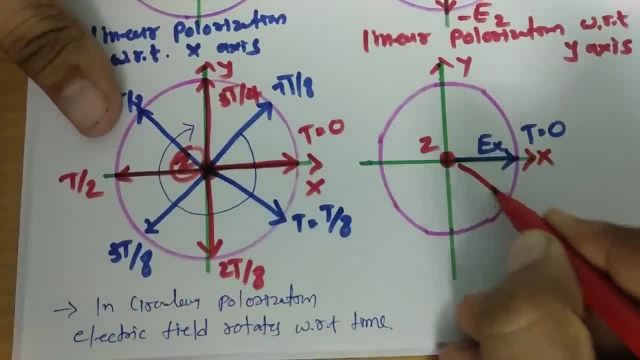 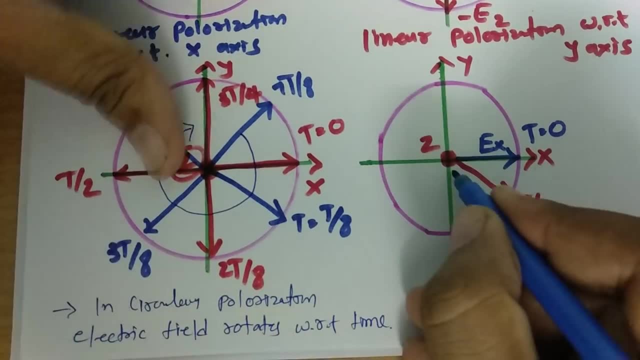 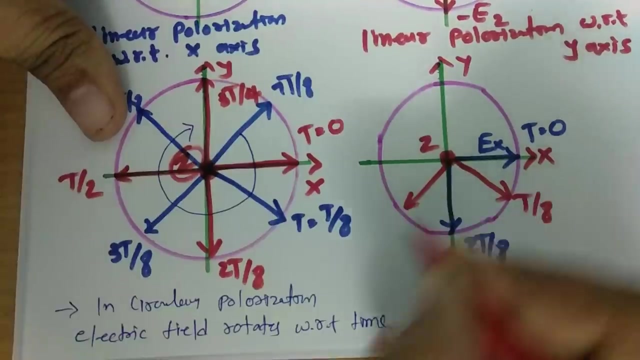 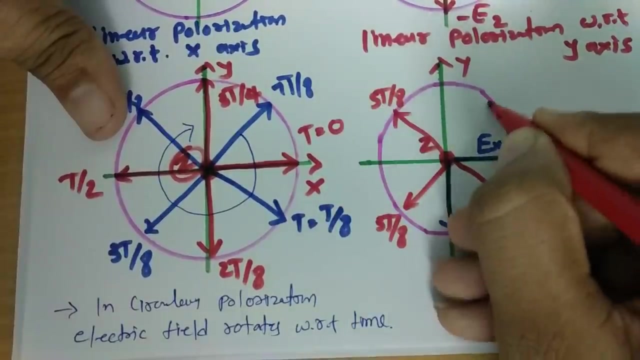 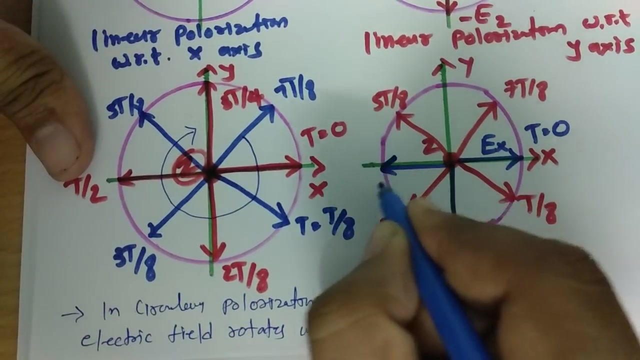 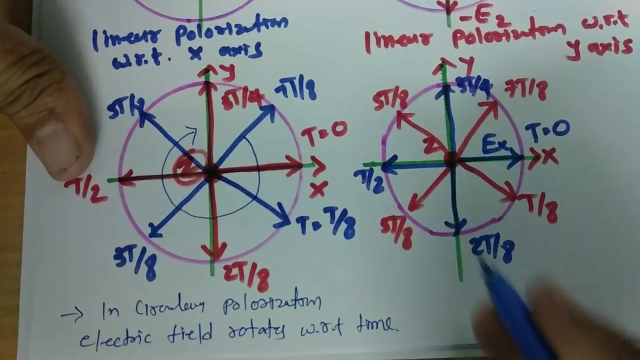 Now, with respect to time, it is revolving, So it is over here after time t by 8.. It is here after time 2t by 8. it will be here after time 3t by 8, over here. after time 5t by 8. it will be over here after time 7t by 8 and after time t by 2. it will be over here. after time 3t by 4. it will be over here. 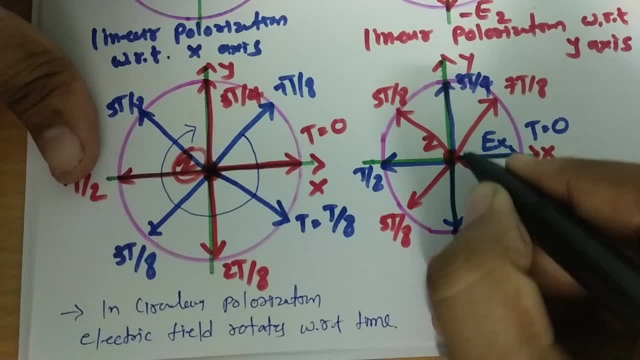 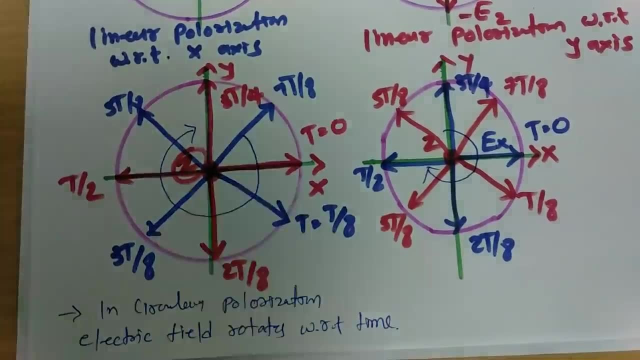 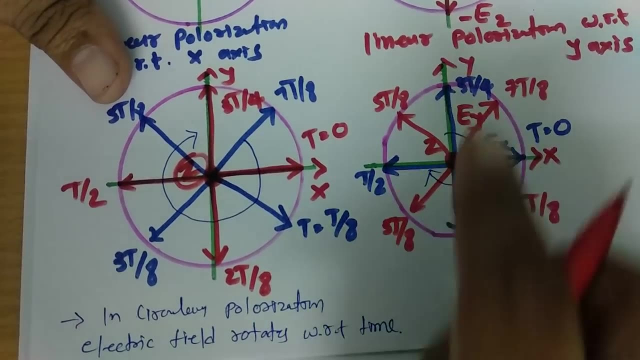 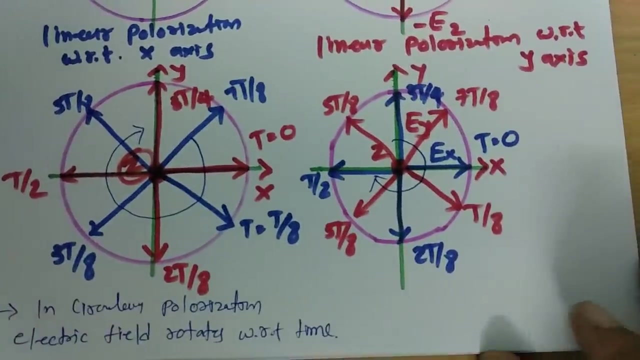 So over here even it is revolving. But the difference is electric field. over x-axis it is e x and over y-axis it is e y. So magnitude over x-axis electric field is different. So this is what. elliptical polarization. So in elliptical polarization 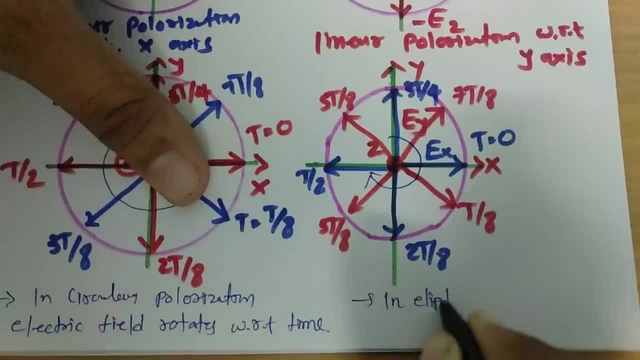 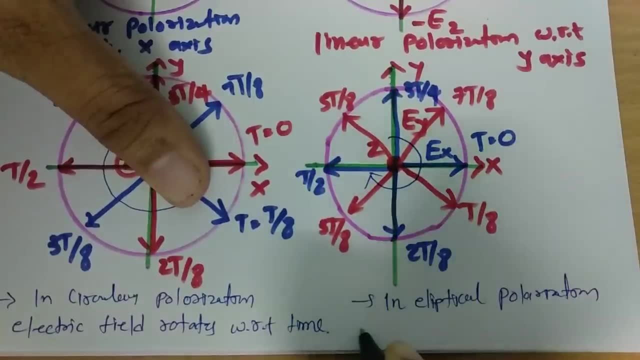 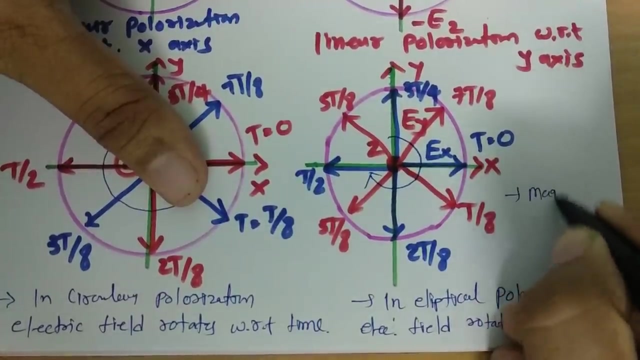 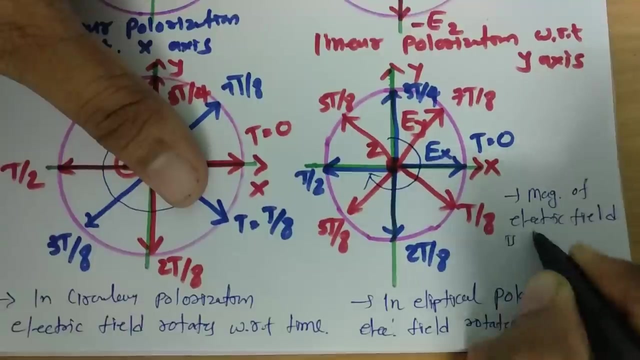 In elliptical Polarization, Electric field Rotates With respect to Time, But the difference is magnitude of electric field. Magnitude of Electric Field Is different On X And Y Axis, So that is how it is different. 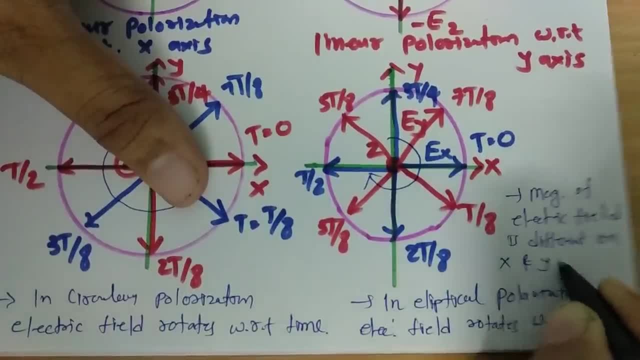 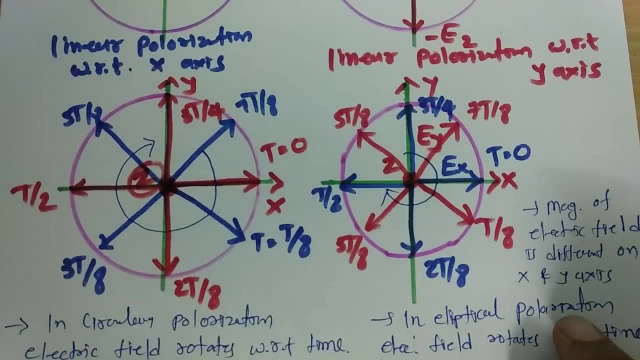 Now, As if I want to say what could be the basic formula of electric field For Circular polarization and for Elliptical polarization, then That is quite interesting. So I have to say, I have to say That, I have to say, 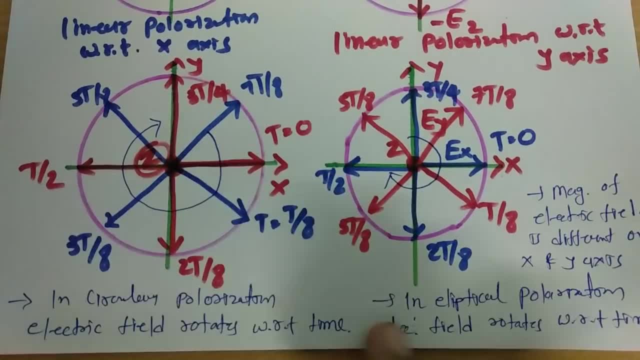 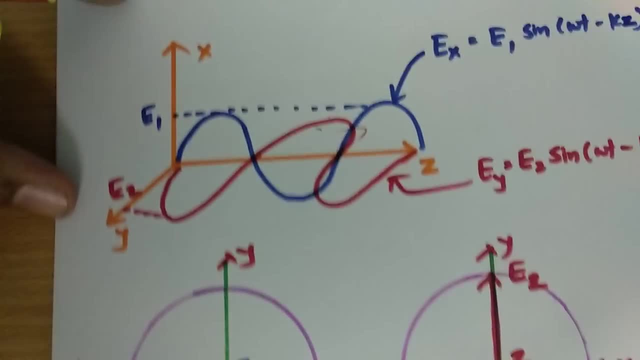 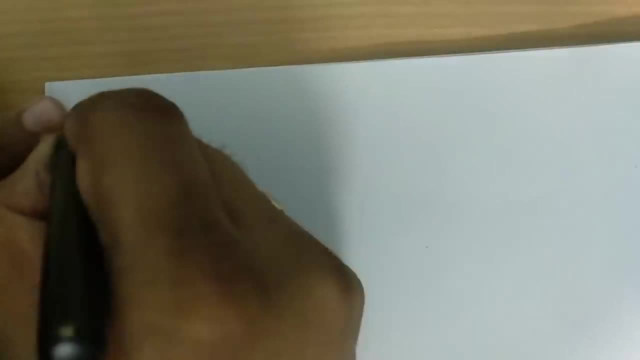 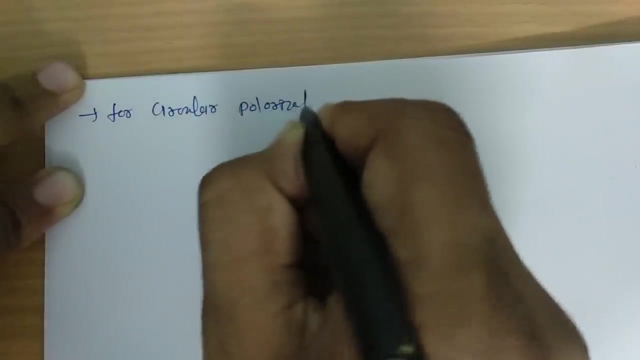 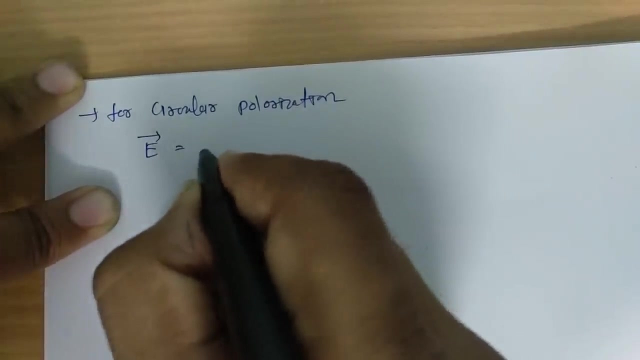 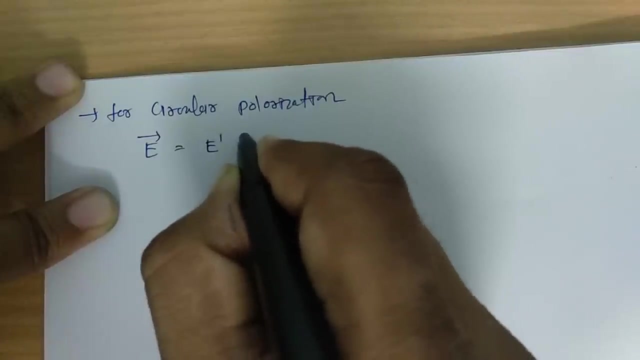 For Circular Polarization. If I say Result In Electric Field That Is E, Then It Will Be E Dash In X Axis, And X Axis Let 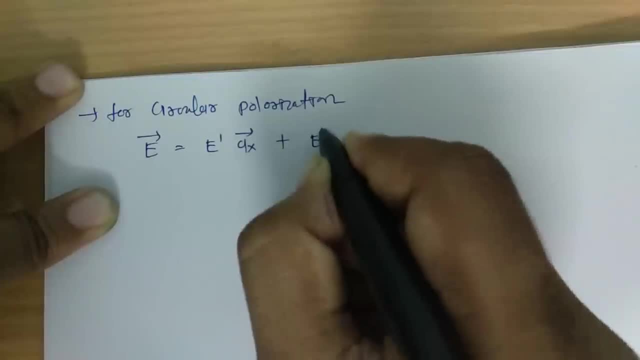 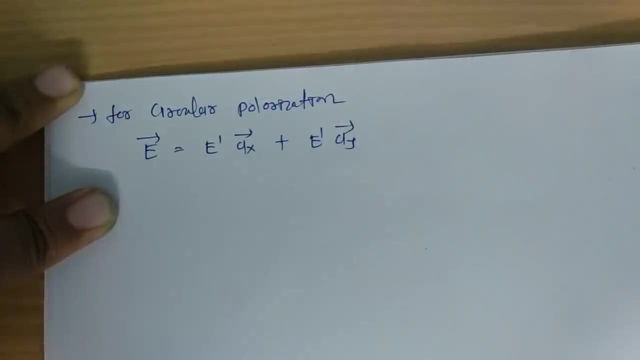 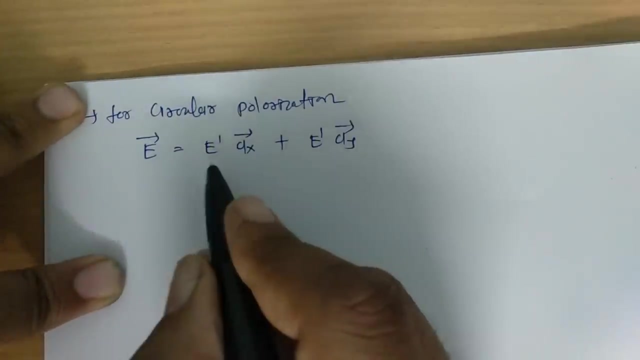 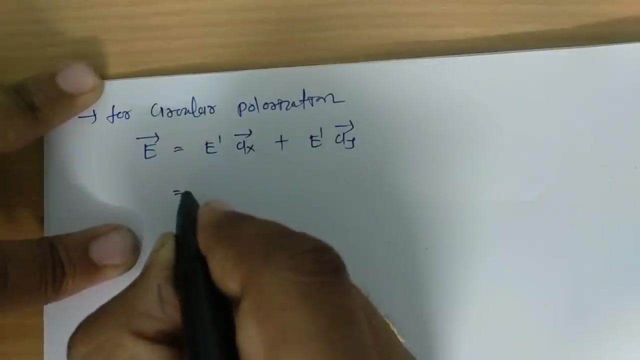 Us Say Ax Direction, Plus It Will Be E Dash In Y Direction, Where E Dash That Is, That Is, Having Same Magnitude Over X. 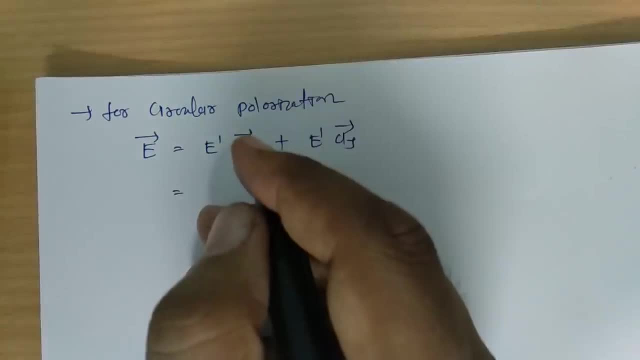 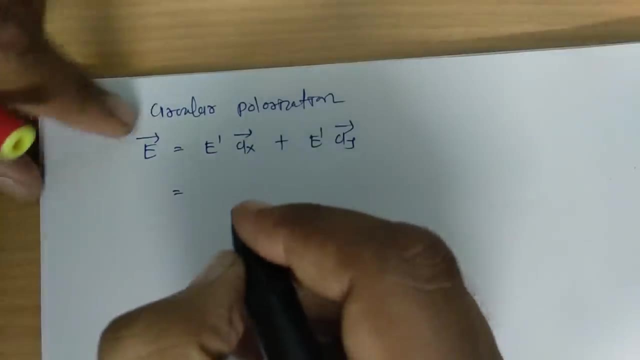 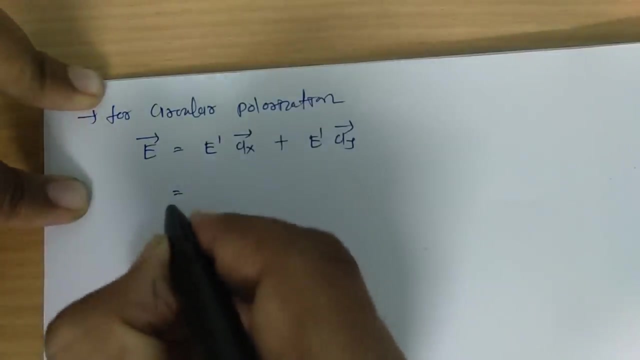 And Formula. So For Circles Formula It's Magnitude That Will Be Like E X Square Plus E Y Square Is Equals To E Dash. 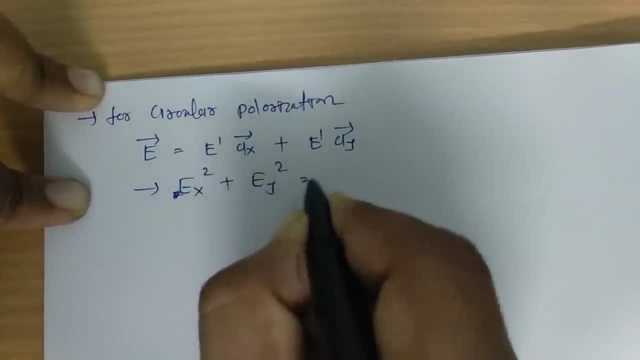 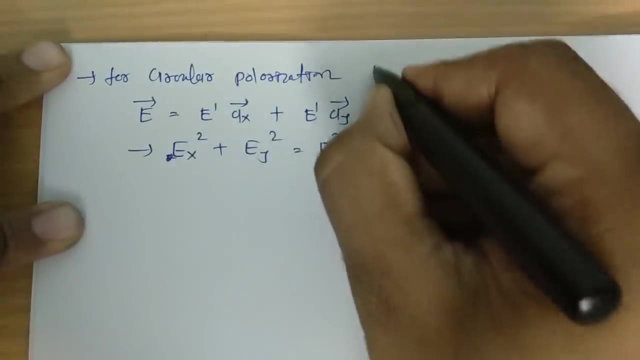 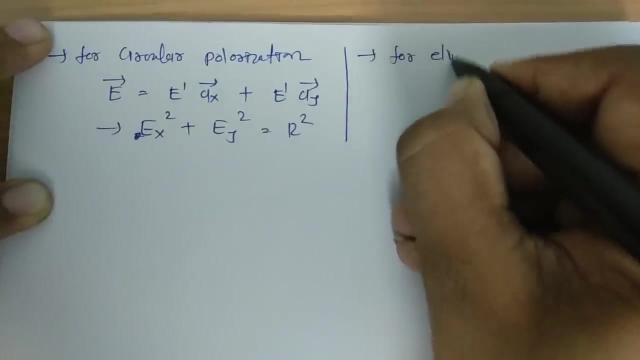 Some Magnitude Square, So Like For R Square. So That Will Happen In Case Of Circular Polarization, While In Case Of Elliptical Polarization 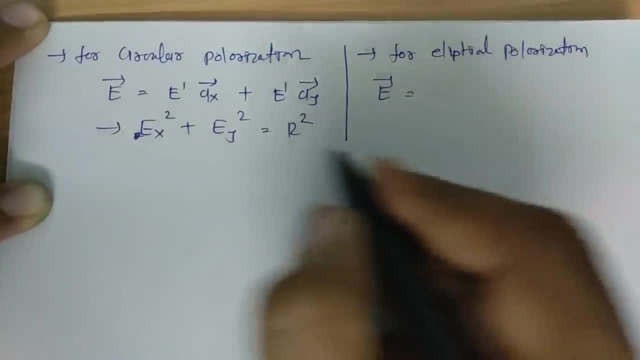 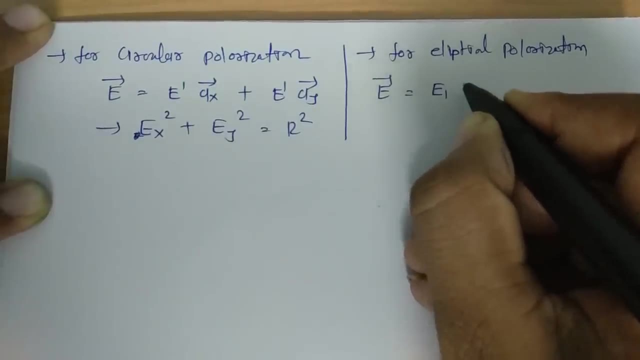 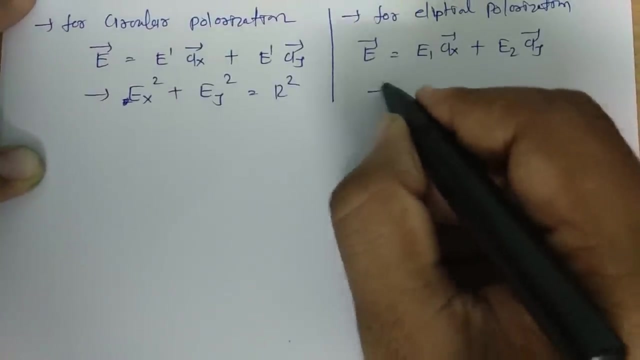 So For Elliptical Polarization Electric Field Magnitude Will Be Different For X Direction And For E 2. In Y Direction, Then It's Basic.